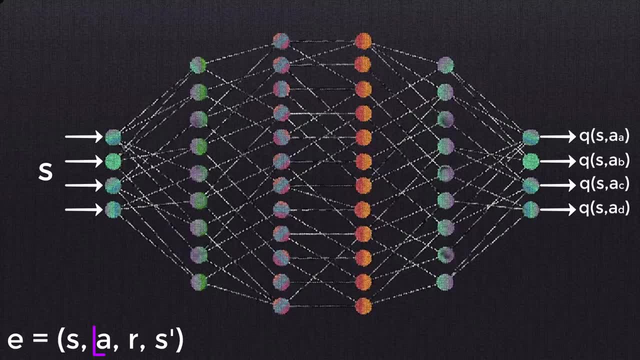 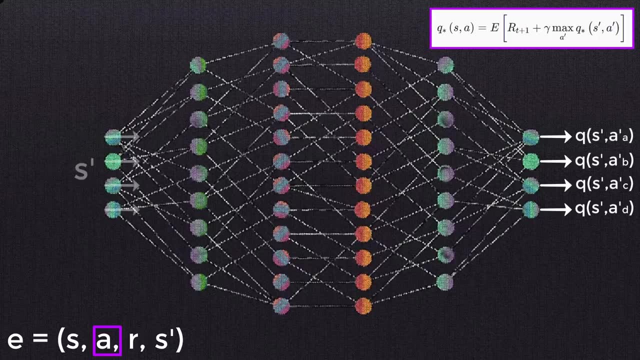 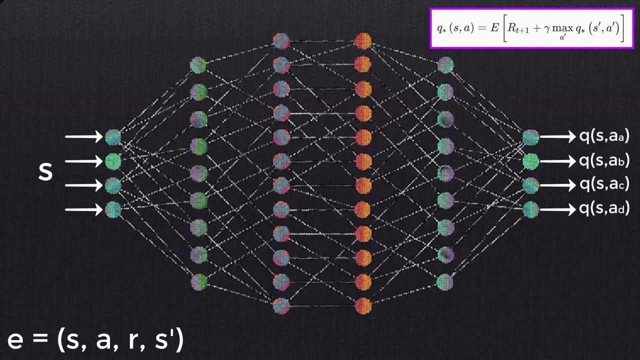 We do the first pass to calculate the Q value for the relevant action and then we do a second pass in order to calculate the target Q value for this same action. Our objective is to get the Q value to approximate the target Q value. Remember, we don't know ahead of time what our target Q value even is, so we attempt. 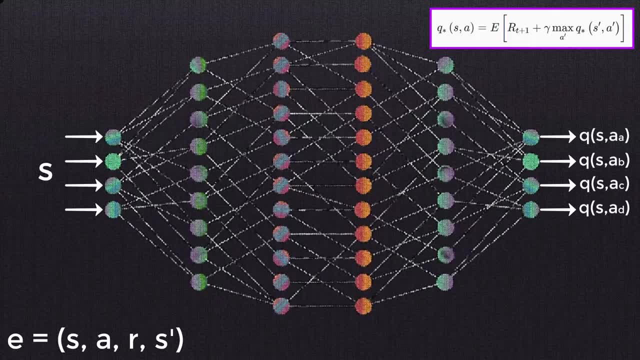 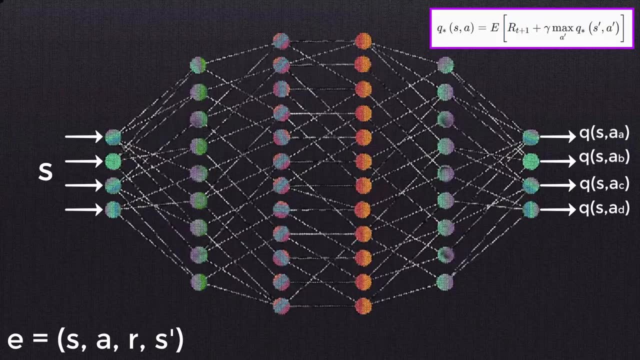 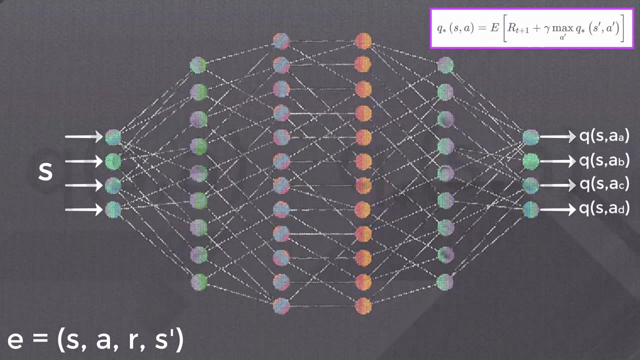 to approximate it with the network. This second pass occurs using the same exact weights in the network as the first pass. Given this, when our weights update, our outputted Q values will update, but so will our target Q values, since the targets are calculated using the same weights. 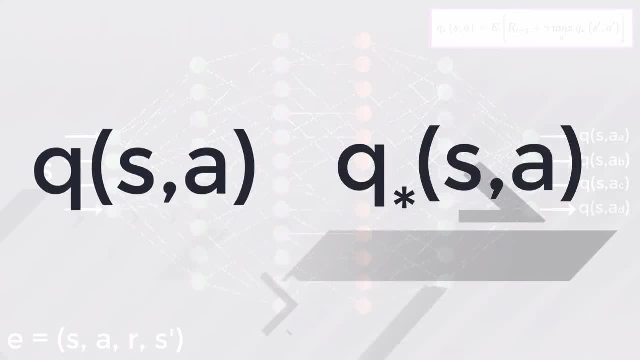 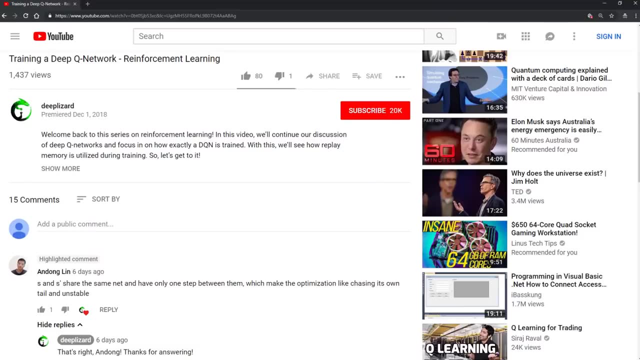 So our Q values will be updated with each iteration to move closer to the target Q values. but the target Q values will also be moving in the same direction. As Ondong put it in the comments of the last video, this makes the optimization process. 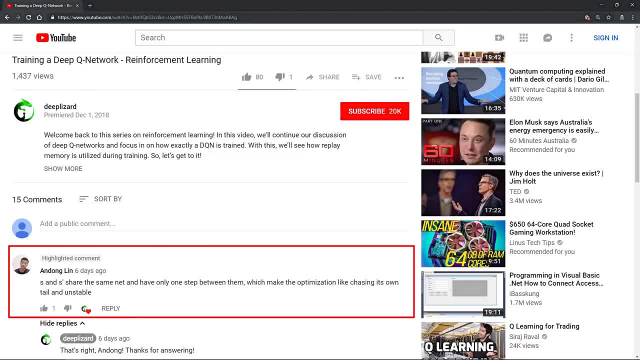 much easier. The optimization appears to be chasing its own tail, which introduces instability As our Q values move closer and closer to their targets. the targets continue to move further and further because we're using the same network with the same weights to calculate both of these values. 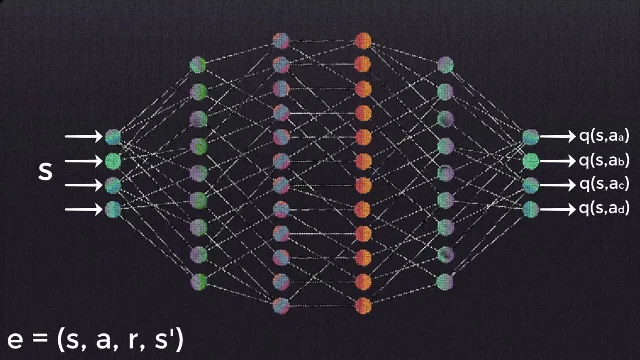 Well, here's a perfect time to introduce the second network that we mentioned earlier. Rather than doing a second pass to the policy network to calculate the target Q values, we instead obtain the target Q values from a target Q value, So in this case we'll call our target Q value targetQValues from a completely separate 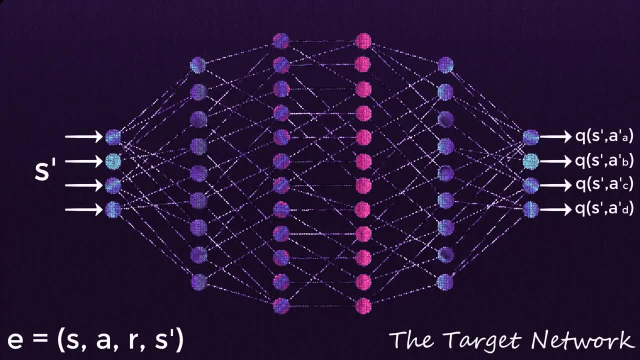 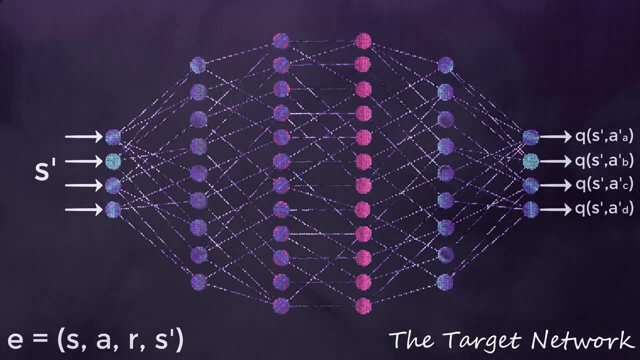 network, appropriately called the target network. The target network is a clone of the policy network. Its weights are frozen with the original policy network's weights and we update the weights in the target network to the policy network's new weights every certain amount of timesteps. 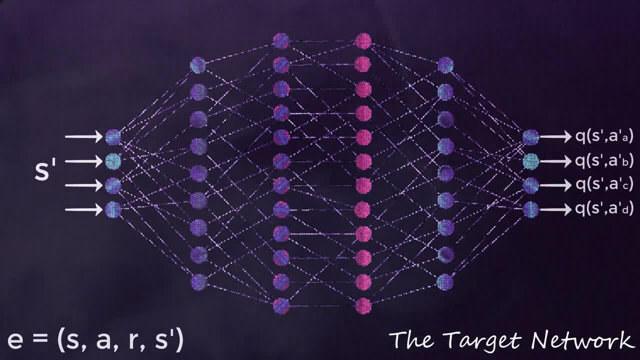 This certain amount of timesteps can be looked at as yet another hyperparameter that we'll have to test in tune to see what works best for us. So now the first pass still occurs with the policy network. Well, that's the end of the video. 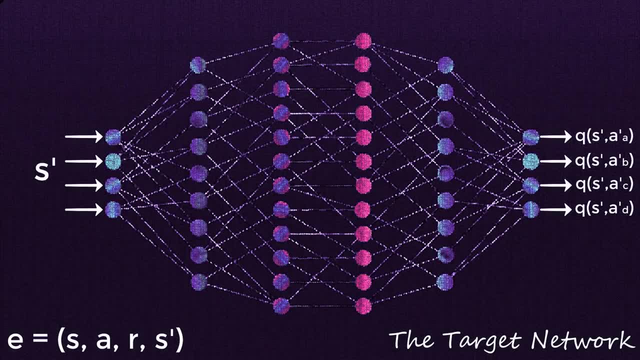 Thank you for watching network. The second pass, however, for the following state, occurs with the target network. With this target network, we're able to obtain the max Q value for the next state and again plug this value into the Bellman equation in order to 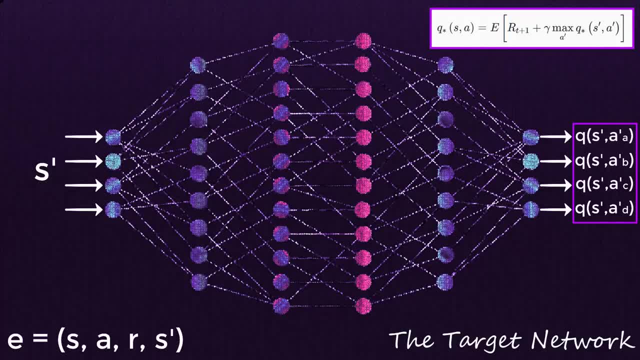 calculate the target Q value for the first state. This is all we use the target network for: to find the value of this max term so that we can calculate the target Q value for any state passed to the policy network. As it turns out, this removes much of the instability introduced by using only one network to 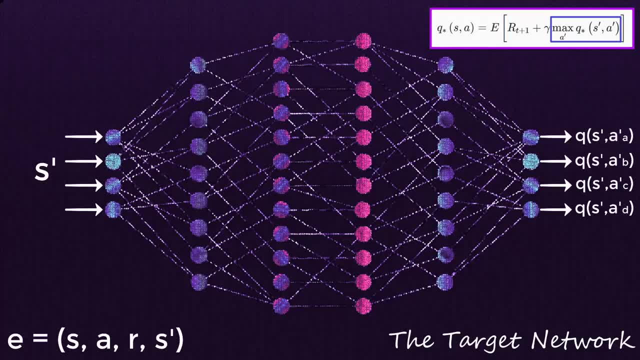 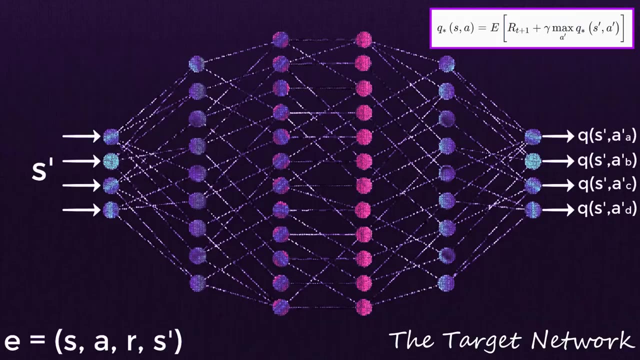 calculate both the Q values as well as the target Q values. We now have something fixed, ie fixed Q targets that we want our policy network to approximate, So we no longer have the dog chasing its own tail problem. Clever fox, As mentioned, though, these values don't. 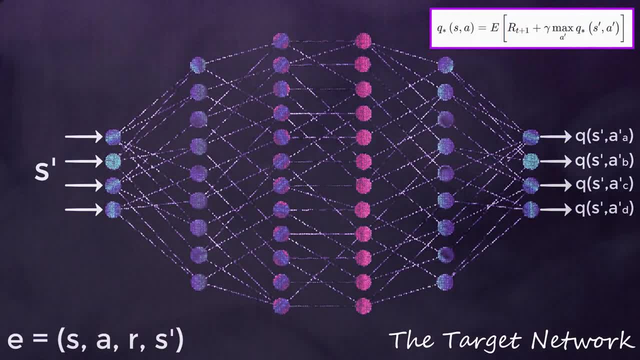 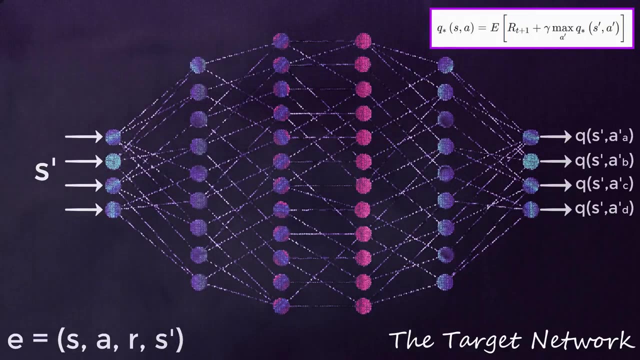 stay completely fixed at the entire time. After X amount of time steps, we'll update the weights in the target network with the weights from our policy network, which will in turn update the target Q values with respect to what it's learned over those past time steps. This will cause the policy network to start to 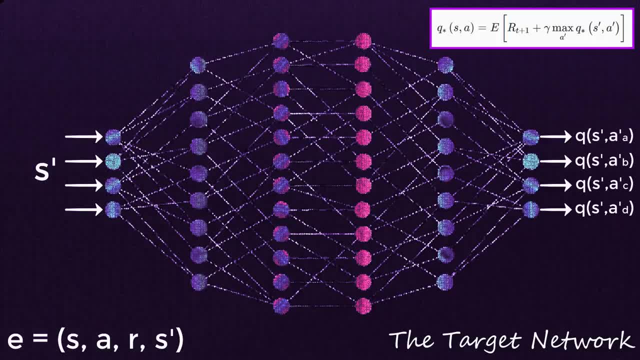 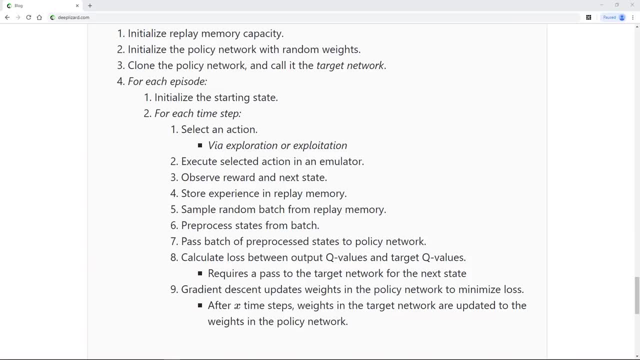 approximate the updated targets. Alright, so now let's just highlight what's changed in our training summary since we've introduced this target network. For the most part, this is all the same. We only have a few tweaks. The first change is that we now have a new step at 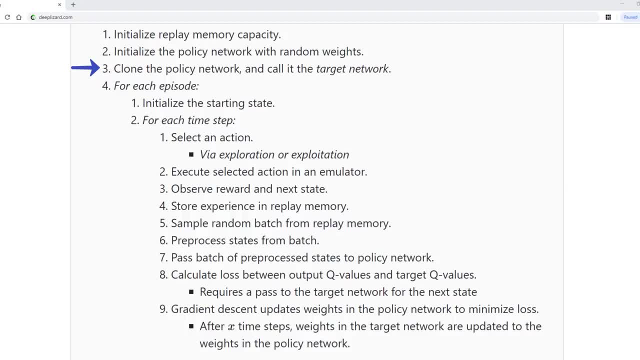 the start where we clone the policy network and call that clone the target network. Additionally, when we calculate the loss between the Q value outputs from the policy network and the target Q values, we do this using the new target network now rather than with a second pass to the policy network, The last. 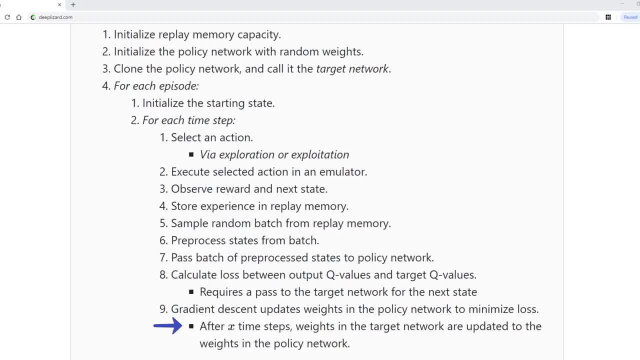 change is just that we update the target network weights with the policy network weights every X time step. Take some time to go over this new algorithm and see if you now have the full picture for how target networks fit into the DeepQ network training process. Let me know your thoughts. 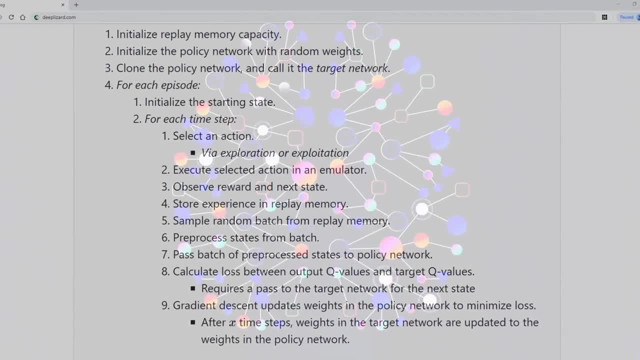 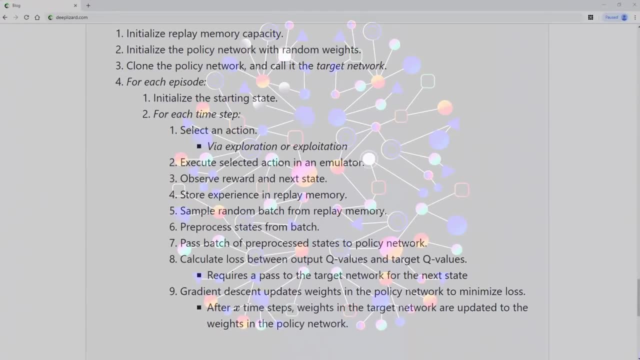 in the comments, And also, please leave a thumbs up to let us know you're learning, and be sure to check out the corresponding blog to this video, as well as the Deep Blizzard Hivemind, for exclusive perks and rewards. Thanks for contributing to Collective Intelligence and. 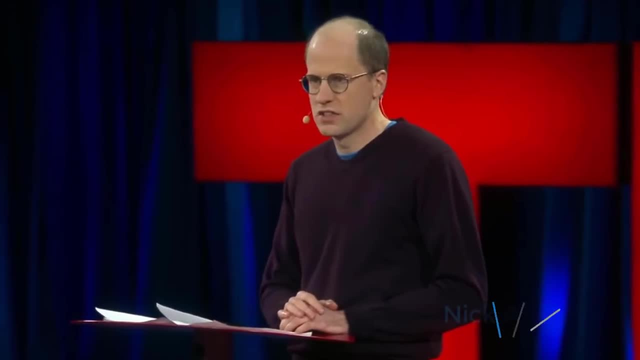 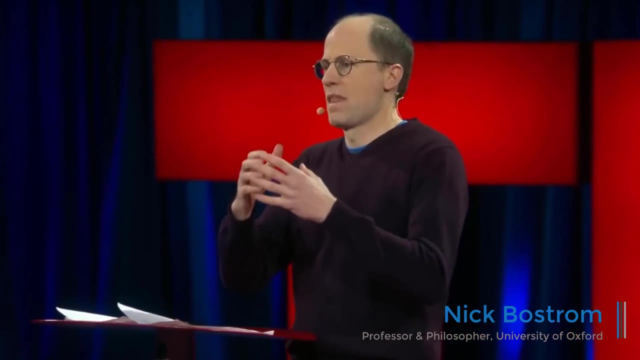 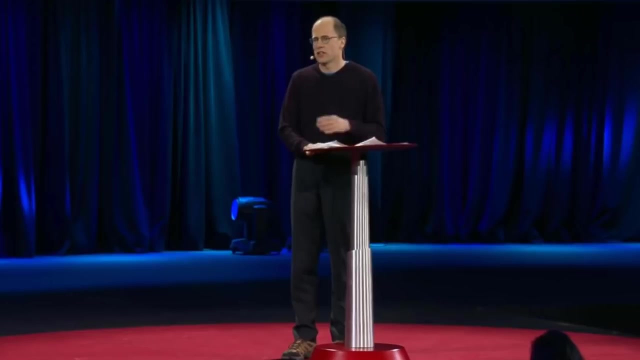 I'll see you in the next one. A paradigm shift has taken place in the field of artificial intelligence. Today, the action is really around machine learning. So, rather than hand crafting knowledge, representations and features, we create algorithms that learn, often from raw perceptual data.